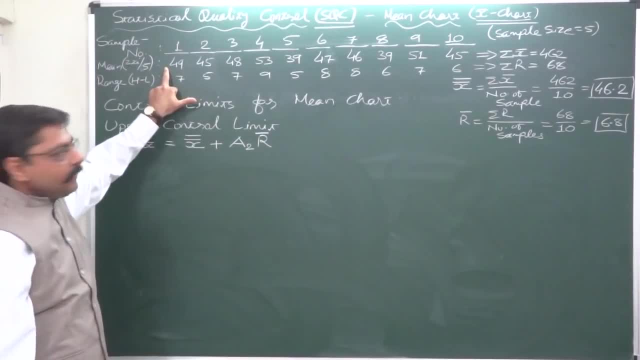 sigma x upon size or n For each and every of the ten samples. the calculation has already been made. This is sigma x for sample one divided by sample size- five. that is common for all samples. This is for second sigma x divided by five, and so on. This is range. 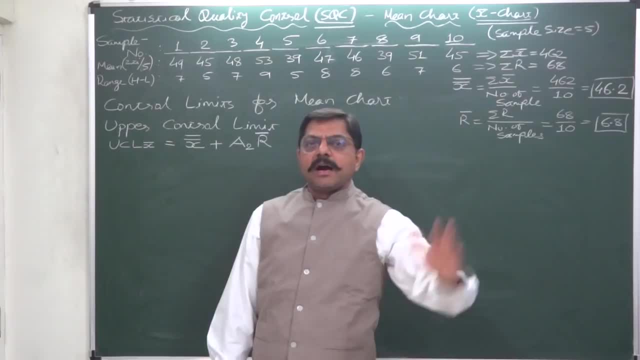 What is range? Range means the difference between the highest value and the lowest value. As we know, sample size is equal to the range of the sample and the range of the sample. So what is range? Range means the difference between the highest value and the lowest value. 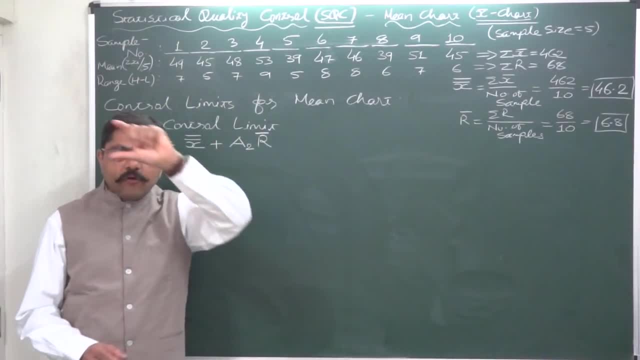 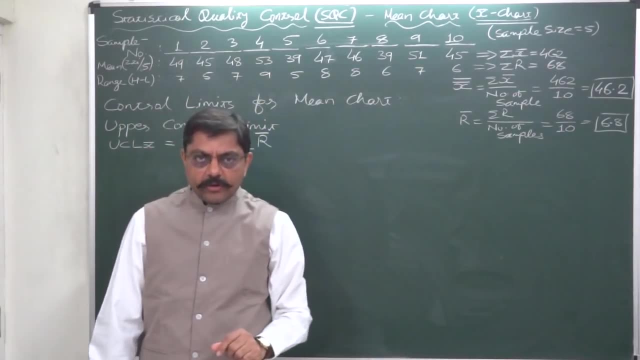 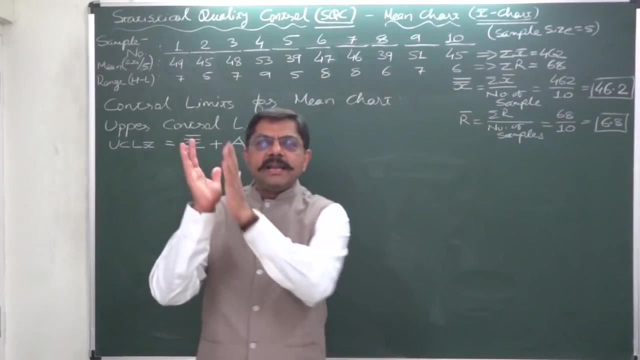 So, for example, if the sample size for each and every sample is five, If all these five sample values or sample points are arranged in ascending order from lowest to the highest for all the five samples, Then we can easily know about the highest sample value and the 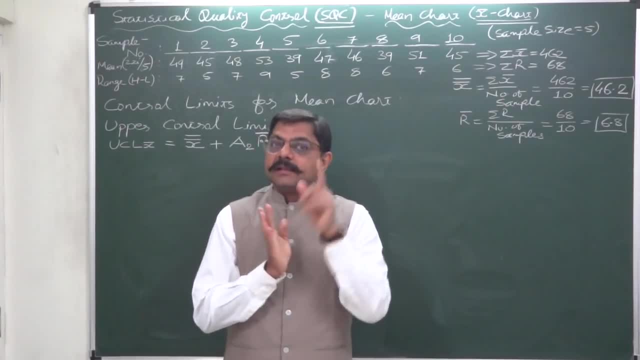 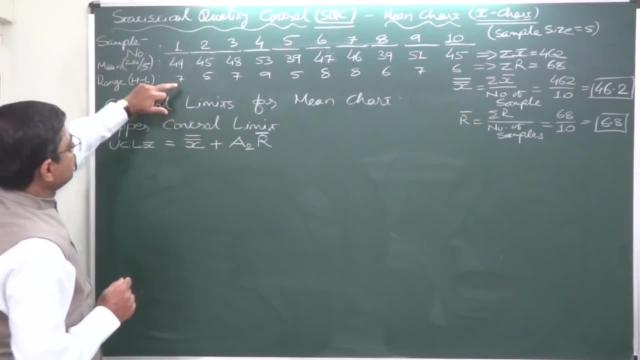 lowest sample value for all the samples. The difference between highest sample value and lowest sample value is known as range. For the first sample, say, it is 7. that means highest sample value and lowest sample value of the first sample. the difference between them is 7, since it is higher minus lower it. 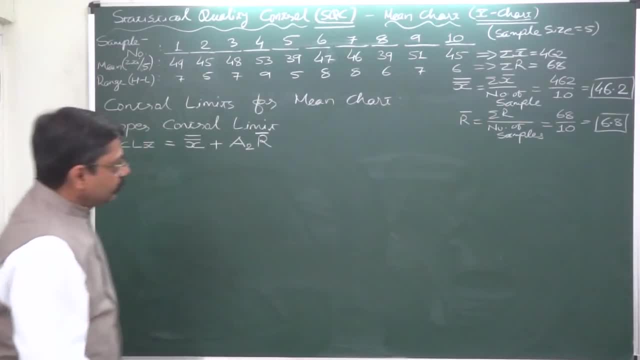 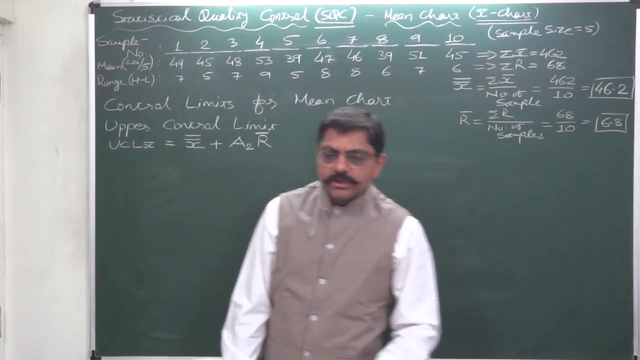 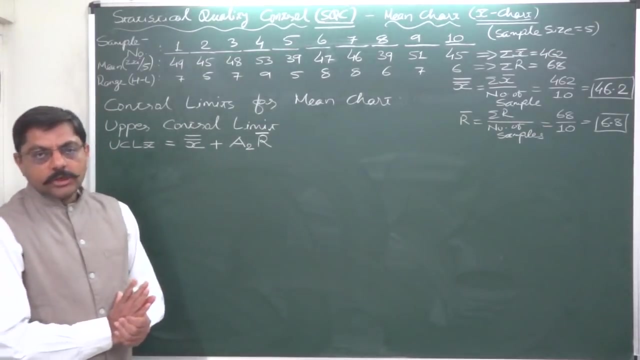 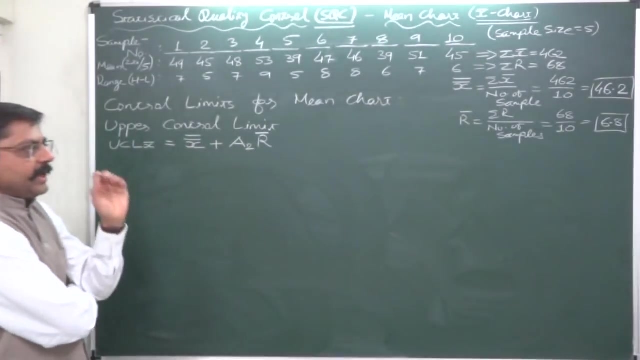 is always positive, so range can never be a negative value. okay, now what to draw any control chart, any type of control chart? we should have upper control limit and lower control limit. to calculate the upper control limit and lower control limit, or say control limits for mean chart, we should have three things. first, 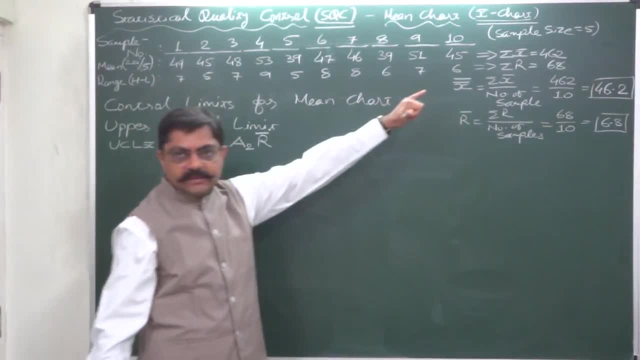 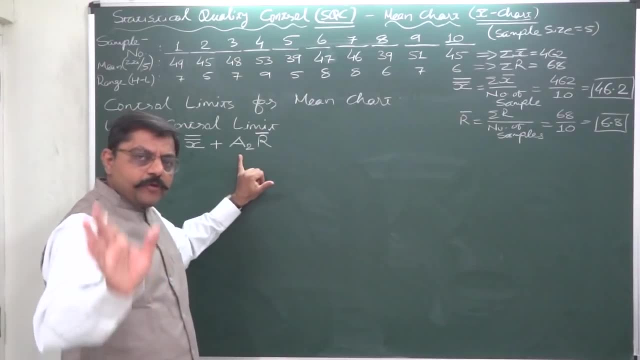 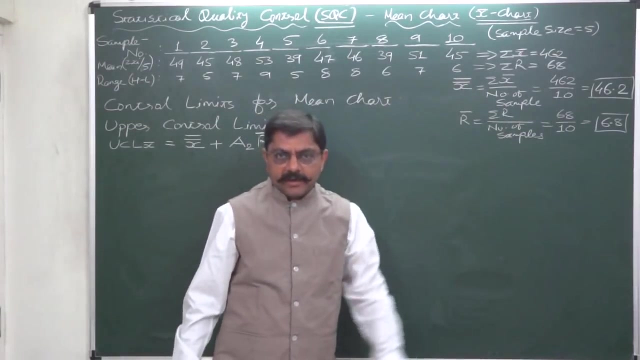 is grand mean. that means mean of all these sample means. so the sign of double bar is there. number two is a to a constant value from a table. it is very easily found. and another is R bar. that is mean of these samples ranges. so I have already calculated the grand mean X double bar. that is nothing. 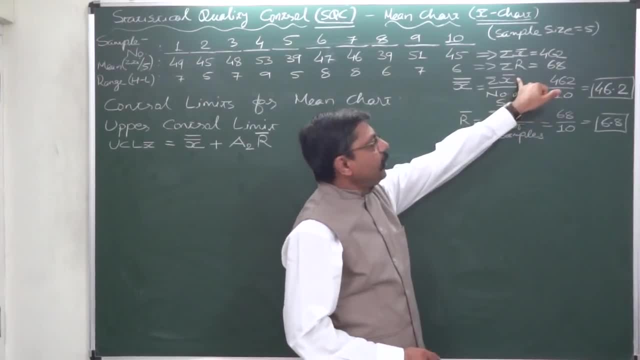 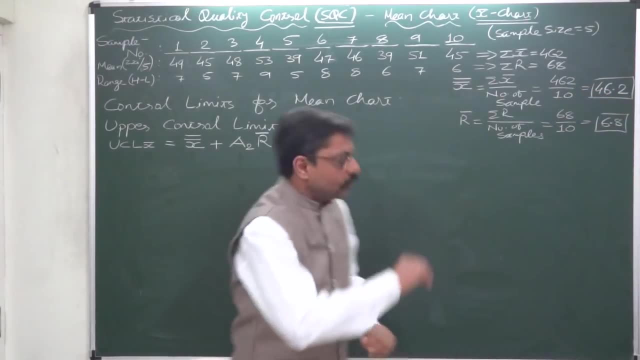 it is mean of all the sample means, that is, summation of all 10 sample means divided by number of samples. it is 462 divided by 10 and it comes to 46.2. similarly, R bar is the mean range, summation of all these ranges, that is. 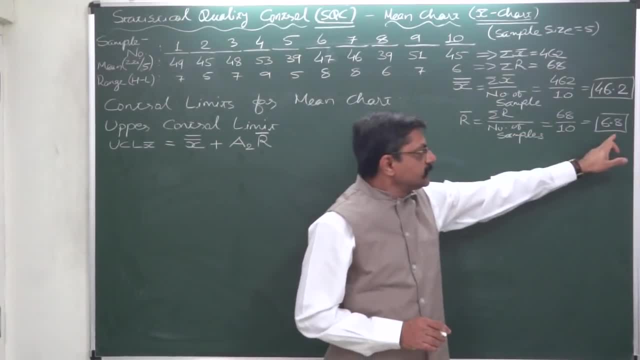 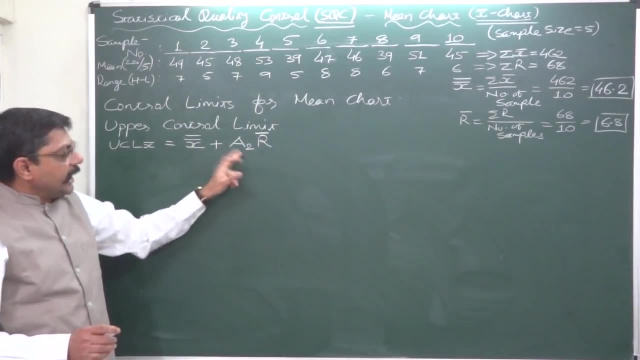 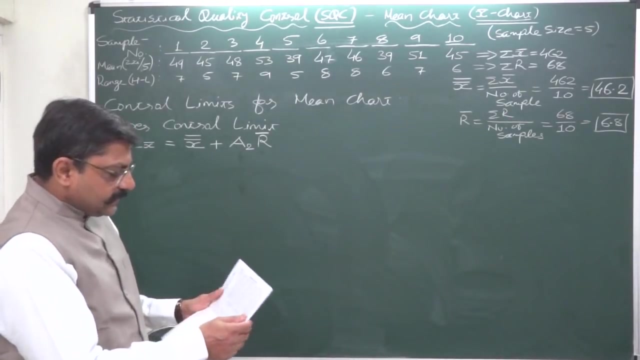 that comes to 68. divided by number of samples, 10, it is 6.8. so these two things are now available to us. how to find out a2? it is available from the statistical tables. in most of the books of statistical Chiavel's it is given mostly. 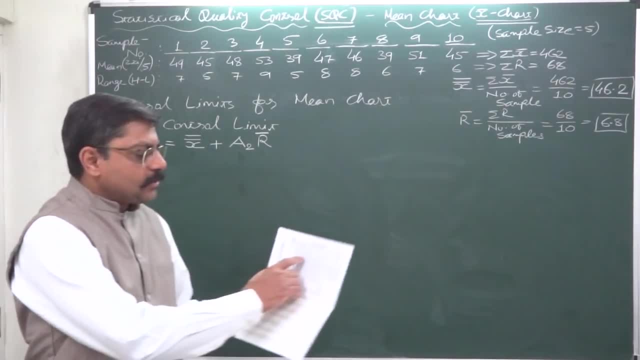 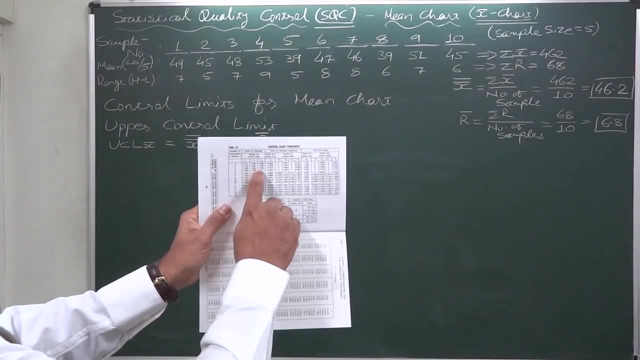 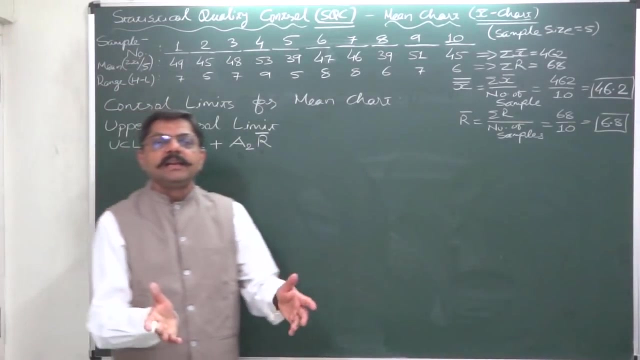 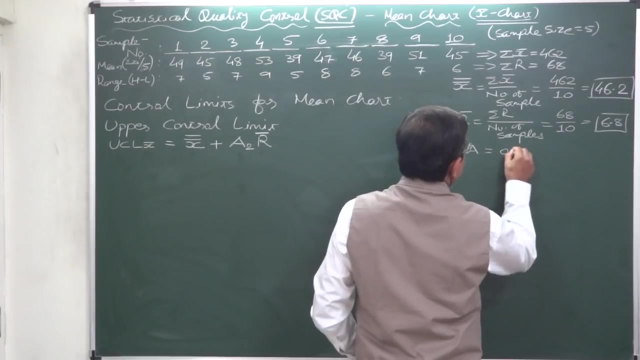 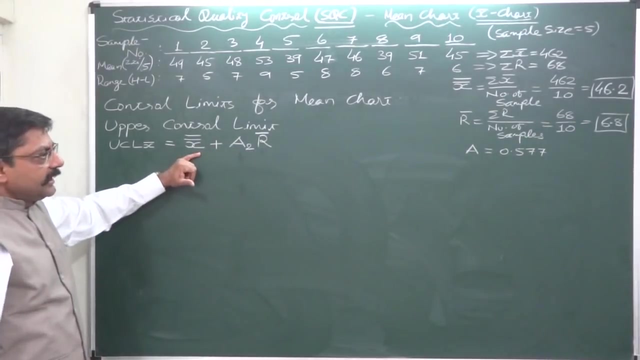 on the last part of the book a2. first of all, size of sample, which is 5 here and for 5 A2 is 0.577.. Many a times paper setters prefer to give it readily in the question, also 0.577.. Okay, So we have all these three ingredients and we can calculate the upper control limit. 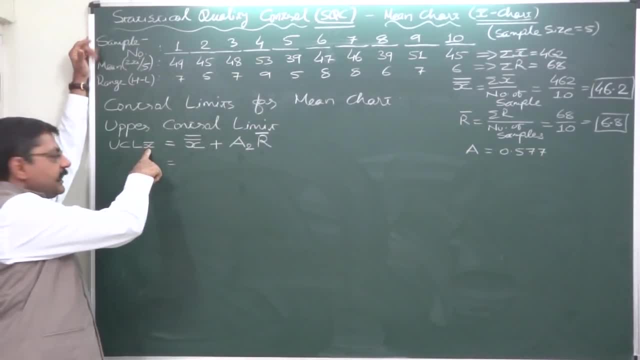 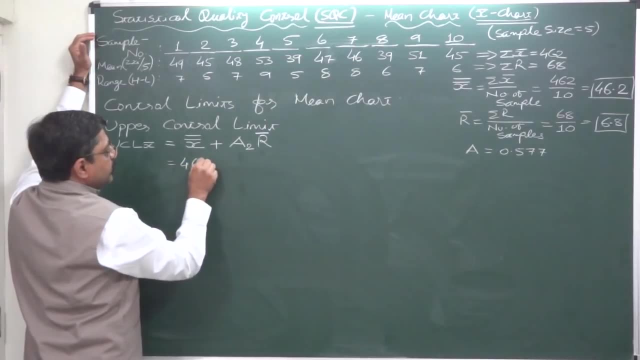 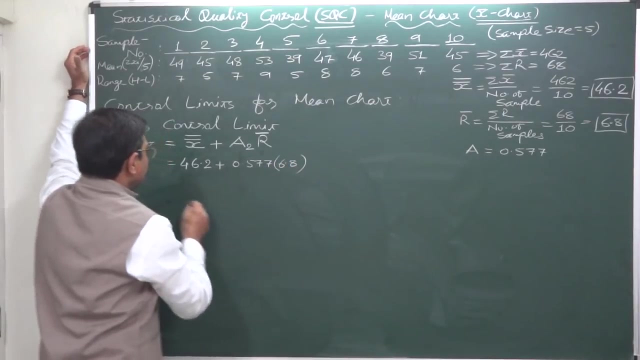 Upper control limit UCL. The X bar in subscript shows that this is the upper control limit for me. chart 46.2 plus 0.577 into 6.8.. That means 46.2 plus 3.9236.. That is 50.1236.. 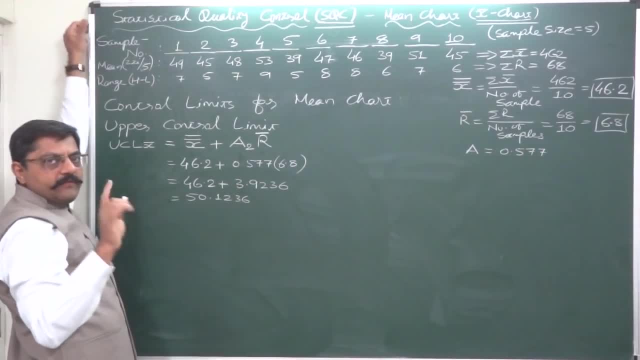 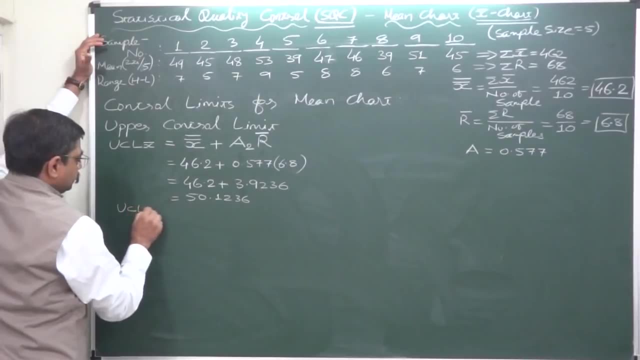 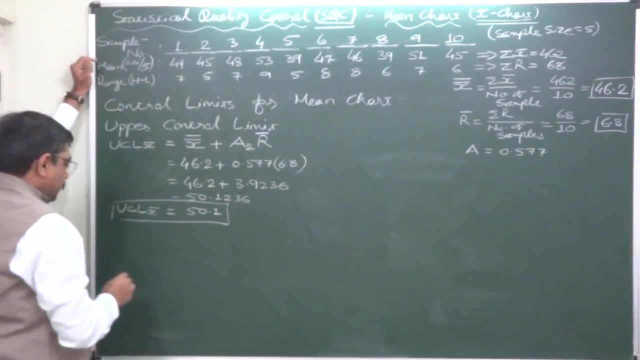 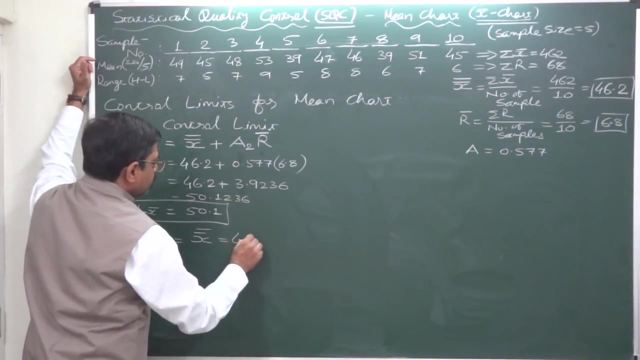 And since we are going to use the graph paper in which we have, say, box trees of 1 millimeter, we are rounding this off to 1 decimal value only: 50.1 approximately. Second will be the central line. That is nothing but grand wing, That is 46.2.. This will be the central line between UCL and LCL. 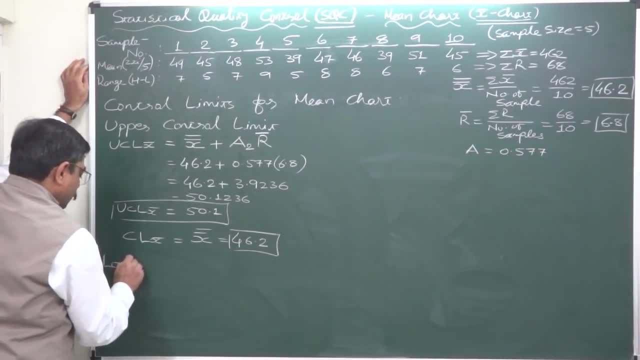 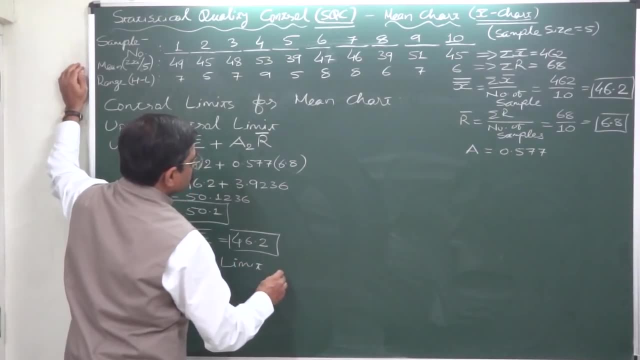 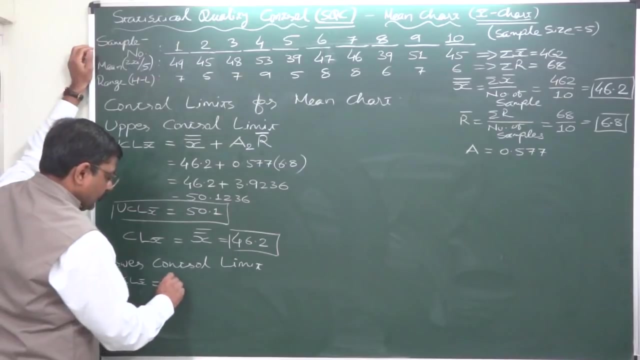 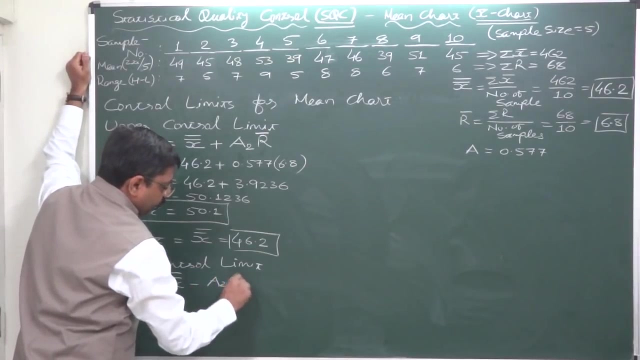 And this is the central line between UCL and LCL. And this is the central line between UCL and LCL. And the third and last thing is lower control limit. Lower control limit, That is called LCL, And since this is for mean chart, it is called LCL X bar. Not much difference between LC and LCL. Grand wing minus A2 R bar. That is the formula. And since we have all the values, it will be 46.2 minus A2 R bar. That is the formula. And since we have all the values, it will be 46.2 minus A2 R bar. That is the formula. 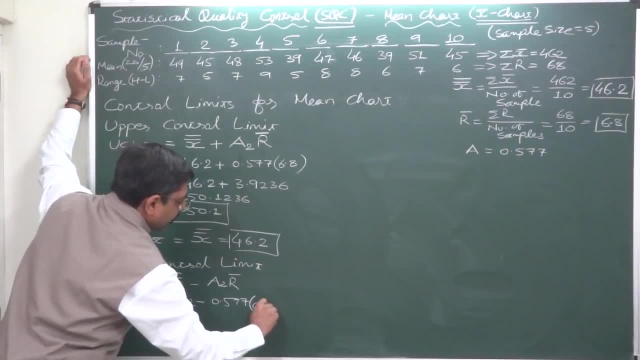 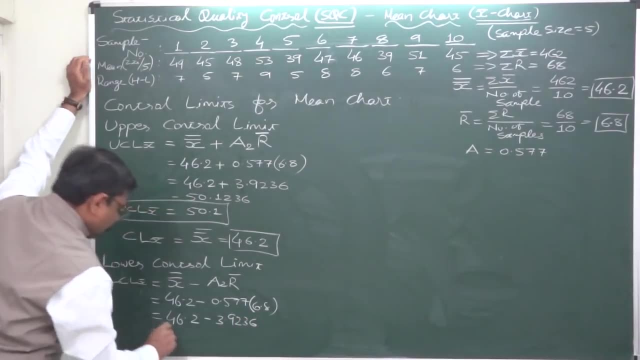 Minus 0.577 into 6.8.. That is 46.2 minus 3.9236.. That comes to 42.2764.. So LCL, the rounded off value for 1 millimeter, comes to 42.3.. 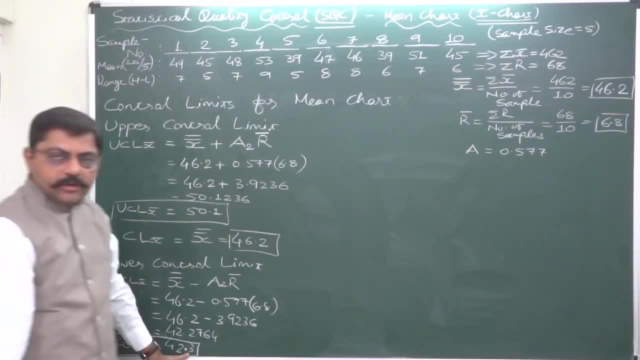 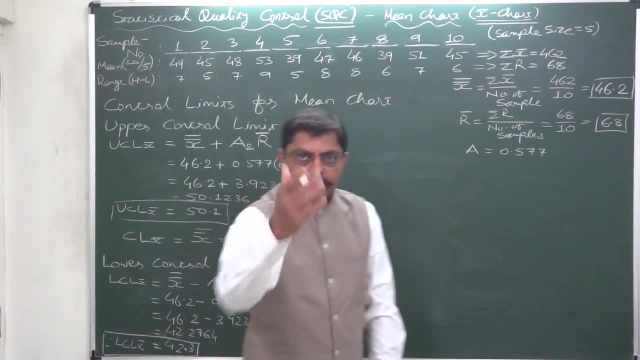 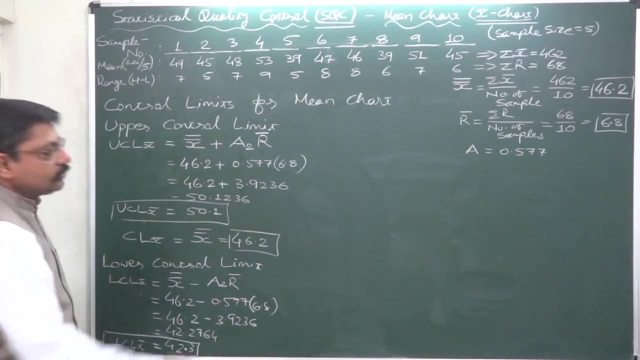 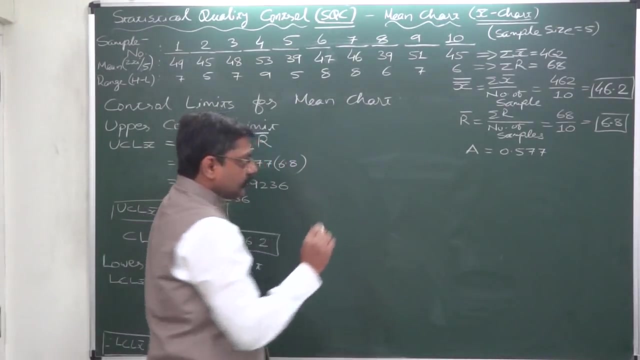 Minus 0.577 into 6.8.. That is the formula And since we have all the values, it will be 46.2 minus A2 R bar. That is the formula And since we have all the values, it will be 46.2 minus A2 R bar. That comes to 42.3.. 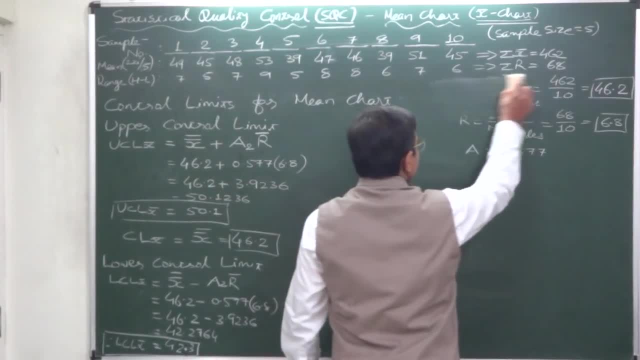 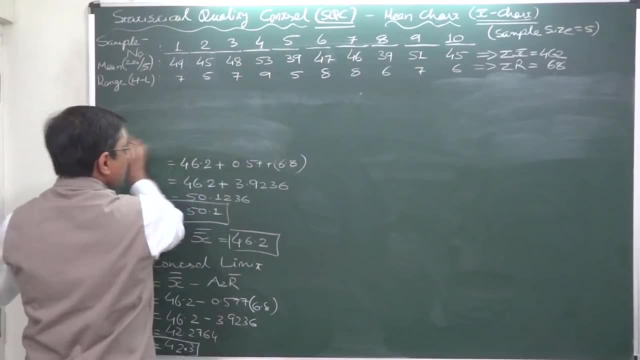 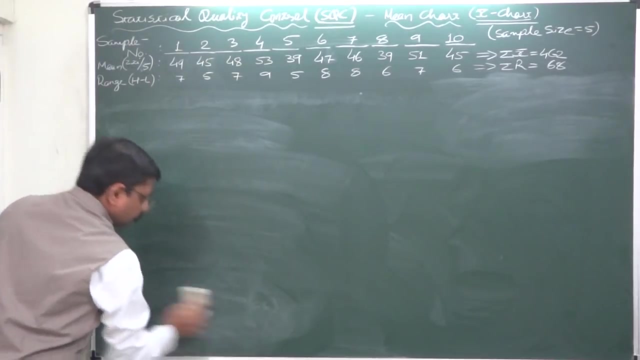 On the graph paper. first draw the x-axis and y-axis. On x-axis, we are going to show the sample number only. On the horizontal axis, we are going to show the sample number only And on the vertical, we are going to show the sample means. 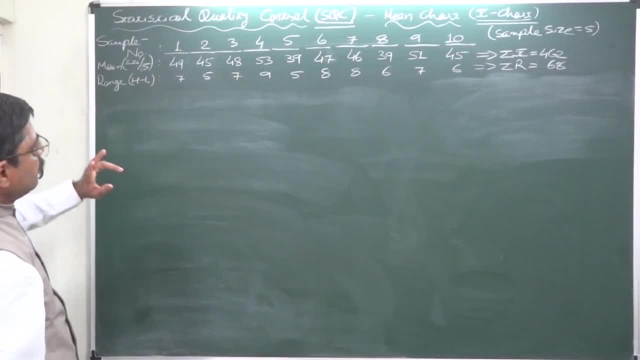 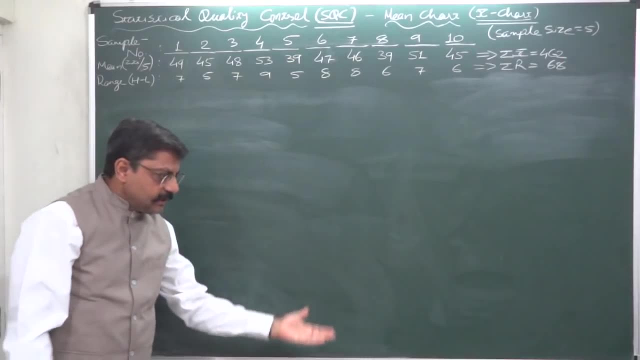 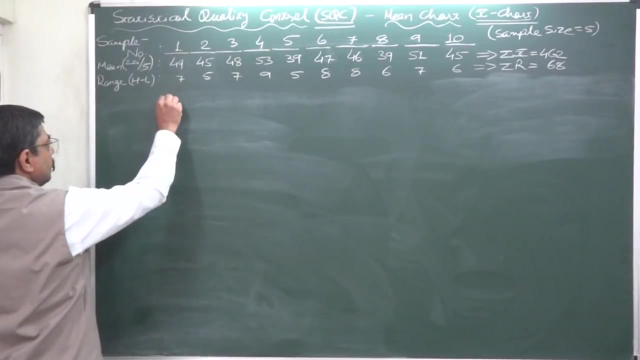 But here the lowest value is 39 and the highest value is 53.. So it is not necessary to start the graph right from 0,, 1,, 2,, 3,, 4,, 5.. We shall pull the vertical axis like this: 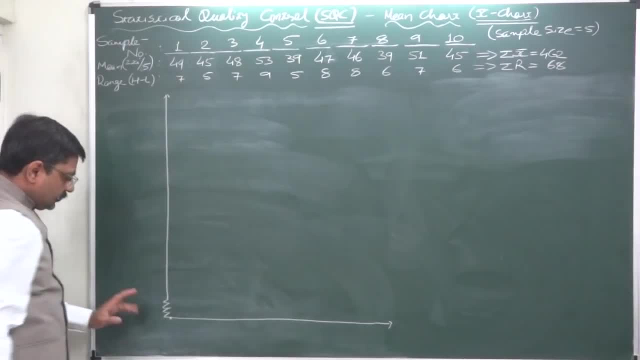 This is called pulling. So we can. We can start with a greater value and then we can maintain the scale Because we need the lowest value. 39 on the graph: Yes, Sample number on horizontal, or popularly known as x-axis, And here sample means. 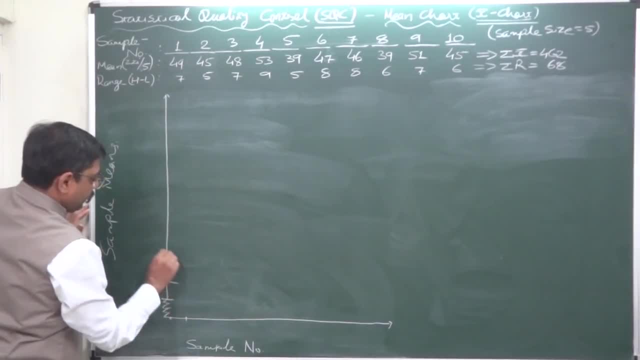 Okay, 39.. 40,, 41,, 42,, 43,, 44,, 45,, 46,, 47,, 48,, 49,, 50,, 51,, 52, and 53.. That is the highest value we need on the graph paper. 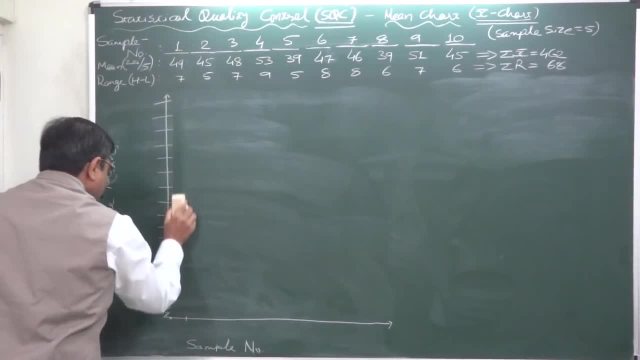 Okay, Yes, As I have already told you, while solving the LPP linear programming problems through graphic method, on this kind of board I am able to draw a sketch. only You need to take utmost care while You need to take utmost care while 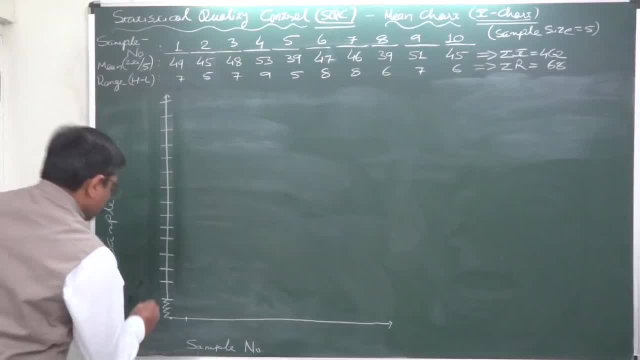 preparing any kind of graph or chart. This is 39,, 40,, 41,, 42,, 43,, 44,, 45,, 46,, 47,, 48,, 49,, 50,, 51,, 52, and 53.. And sample number 1,, 2,, 3,, 4,, 5,, 6,, 7,, 8,, 9, and 10.. Yes, Just Take care of 1 for 1 sample and 1 for 1 unit. 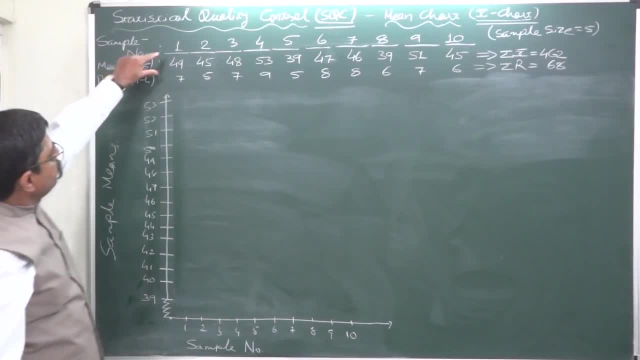 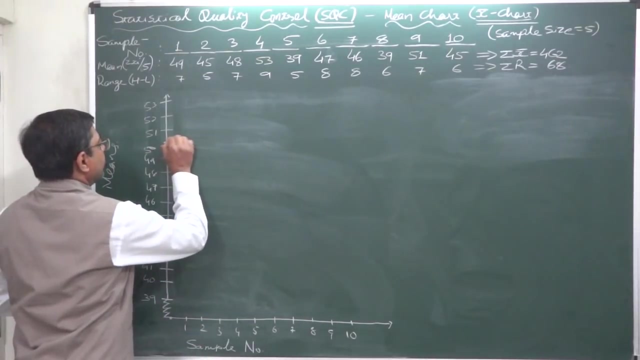 Okay, Now what Just? we need to treat these two as coordinates, But before that we need to draw the control limits. What is the upper control limit? calculated by us, It is 50.1. if we round it off, 50.1 is approximately here: 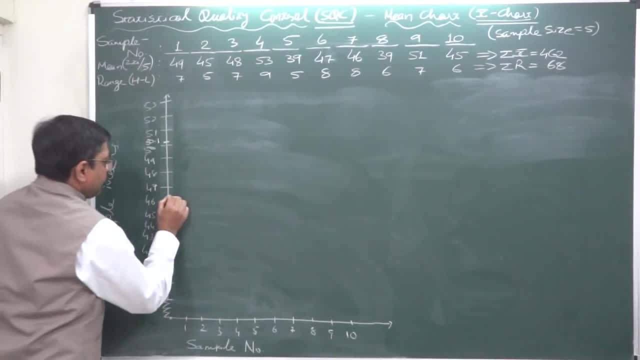 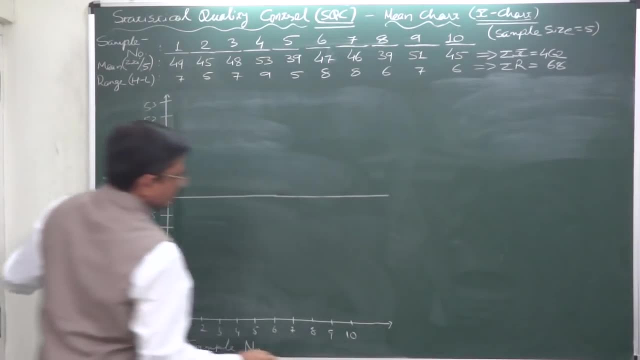 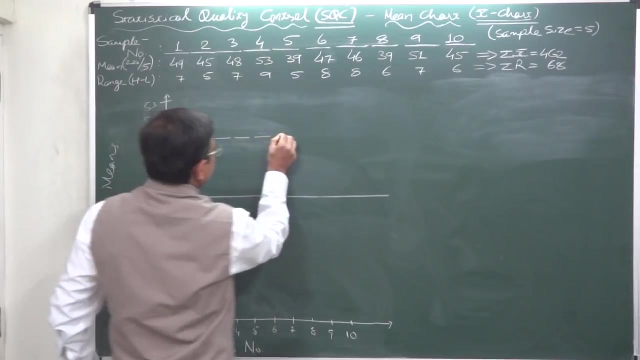 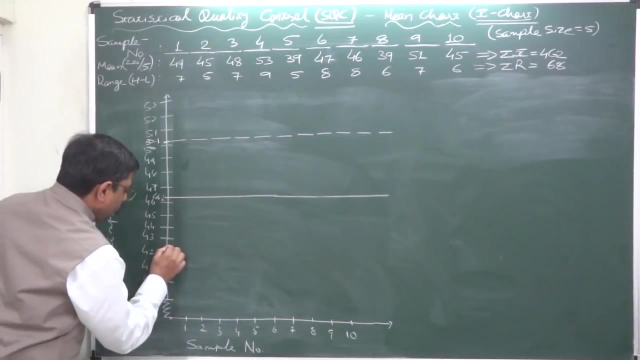 Central limit is 46.2,. it can be here also. Central line is drawn as a continuous line and control limits- upper and lower control limits respectively- are drawn as, say, dotted line, not as continuous lines. Yeah, And lower control limit was 42.3.. 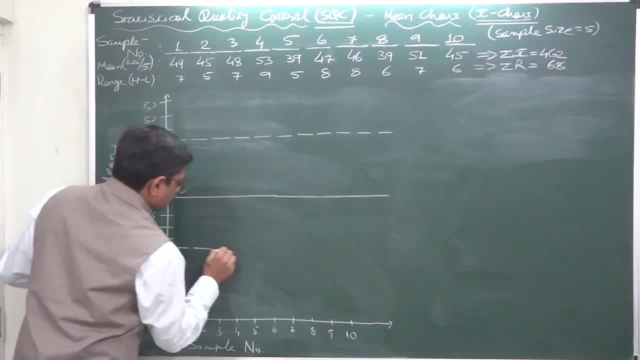 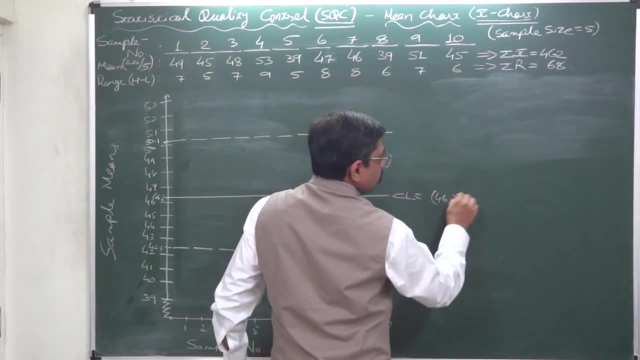 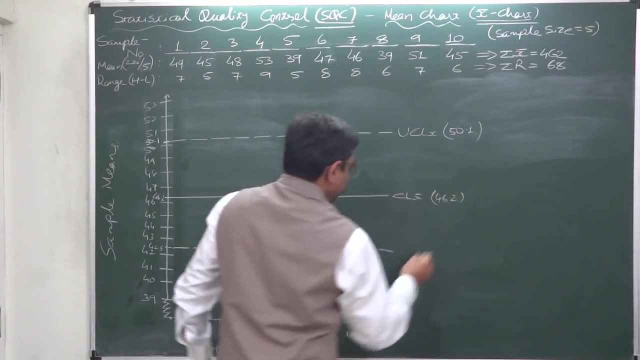 Okay, Okay, Okay, Okay. Okay, We have this as a deadline. This is central line X bar 46.2.. This is upper control limit of X bar, that is 50.1, and this is lower control limit for. 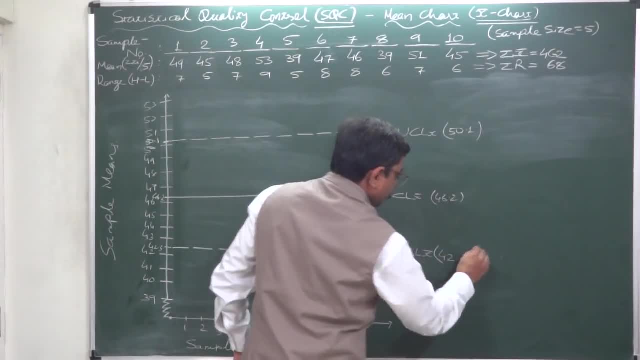 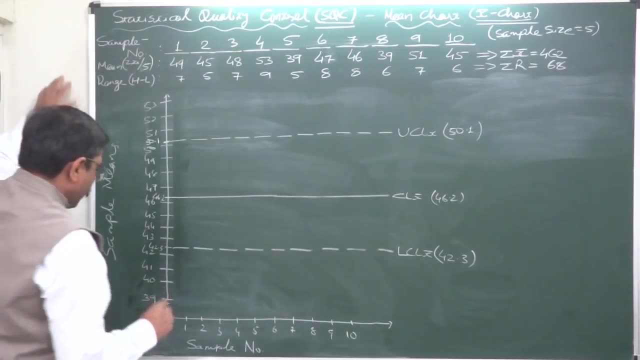 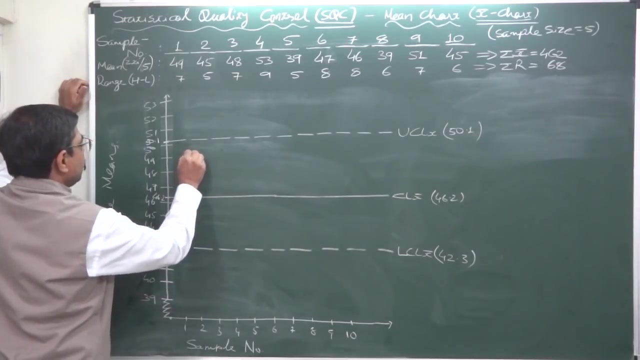 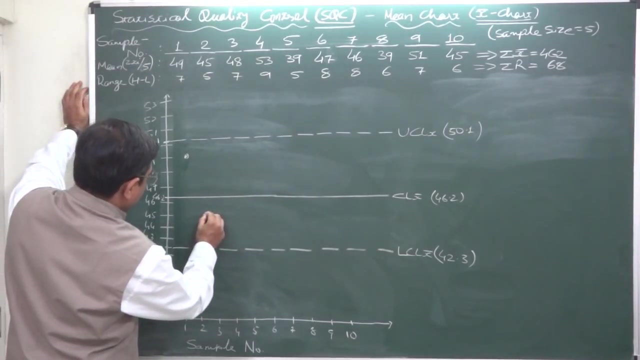 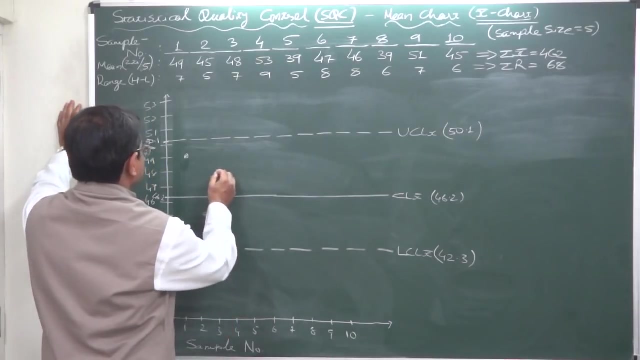 X bar, that is 42.3.. Now we just need to treat these two as coordinates and plot the sample points. For first sample, the sample mean is 49. Yeah, okay, 49, highlighted with a circle. for second, it is 45. for third sample, it is 48. for fourth, 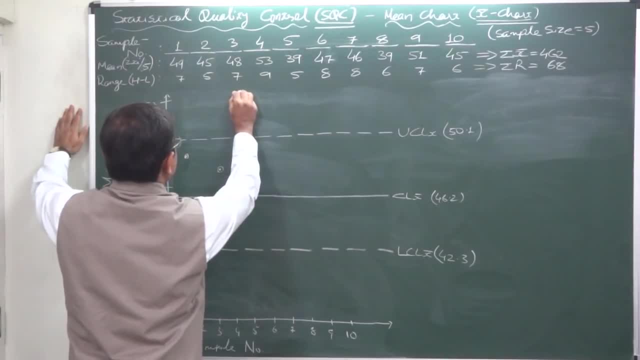 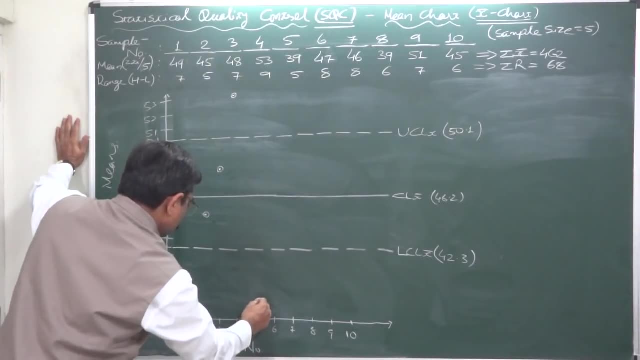 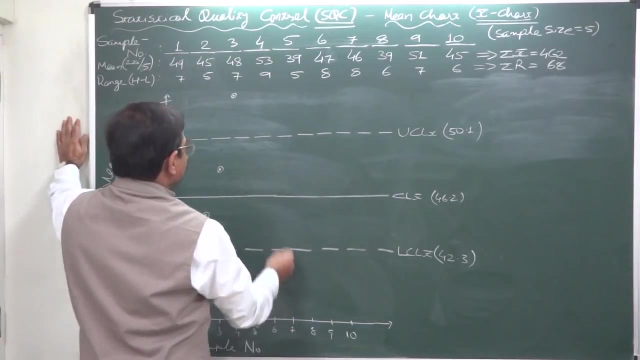 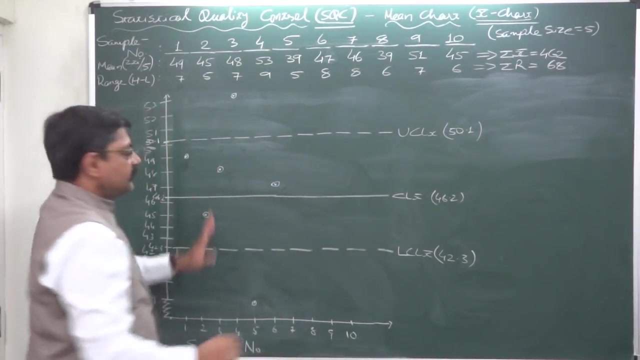 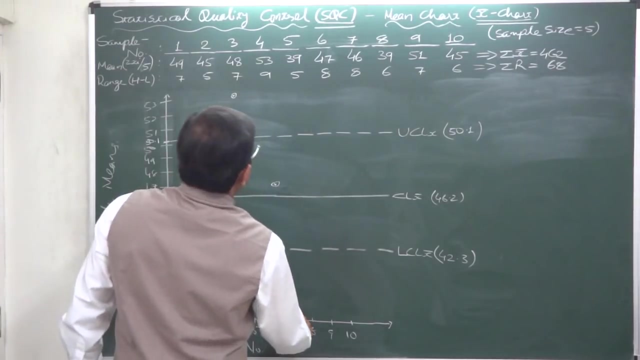 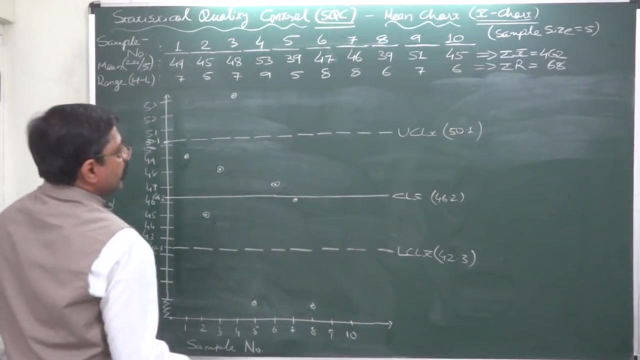 sample, it is 53, the highest value on the chart. for fifth, it is 39, the lowest, see the range of the variation. for sixth, it is 47. this is actually a sketch only. please take utmost care while plotting. for seventh, it is 46 here somewhere. for eighth, it is again 39. for ninth, 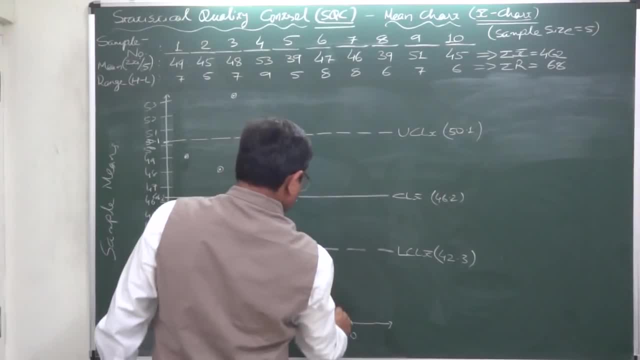 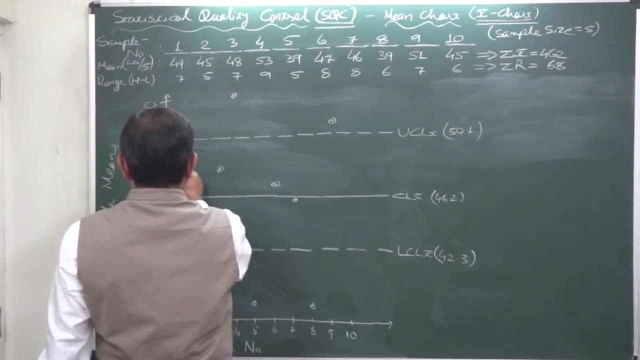 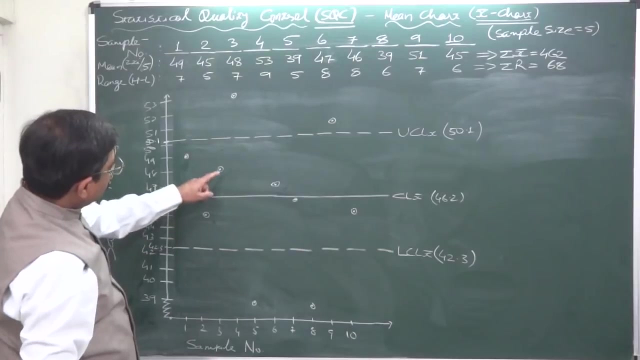 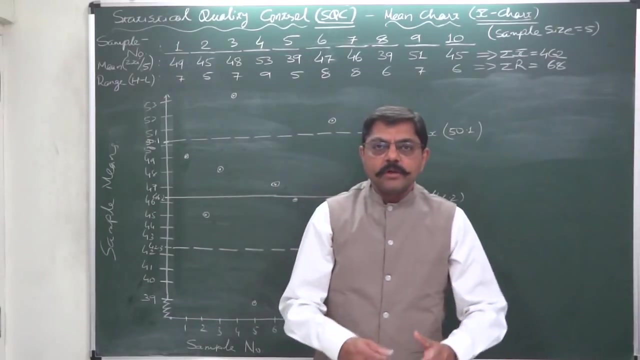 it is 51 and for tenth it is 45: one, two, three, four, five, six, seven, eight, nine and ten. okay, all the ten sample points, or sample means. we have already plotted on the graph now what. it is time of conclusion. but before conclusion, it is time for observation. what is our observation? so? first of all, what we need to observe, or what we. 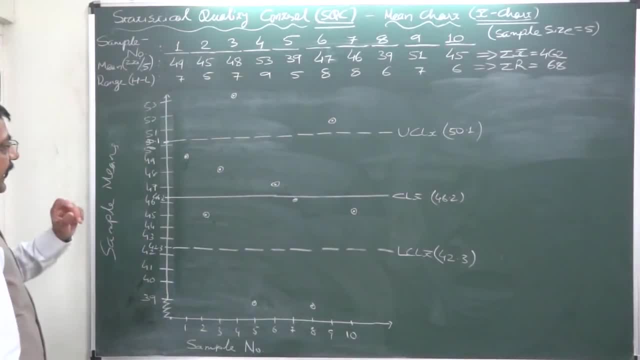 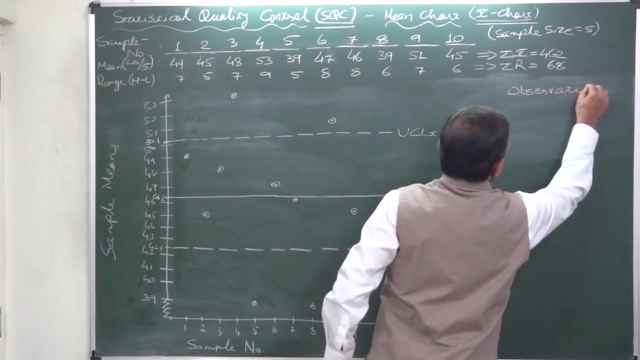 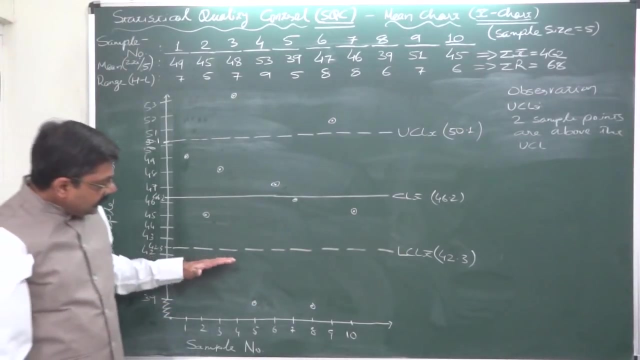 need to check at the time of observation. is there any one or more sample points above the upper control limit? yes, two sample points are above the upper control limit. now it is time of lower control limit. is there any one or more sample point below the lower control limit? yes, there are two. so our second observation for lower control limit is two sample points. it is not necessary to have equal number. no sample point above ucl is possible. no sample point below lcl is also possible. but our aim is to have two sample points below the lower control limit. 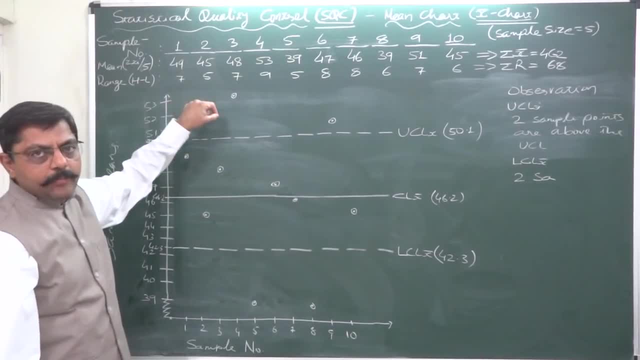 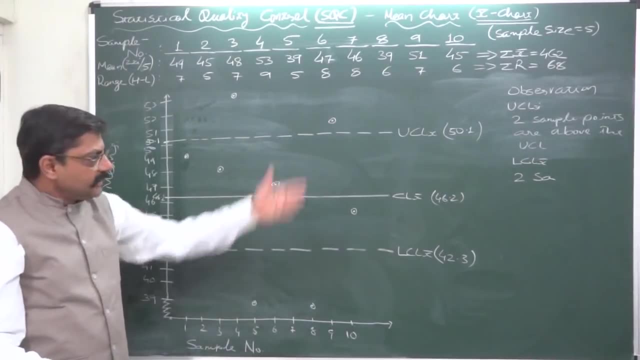 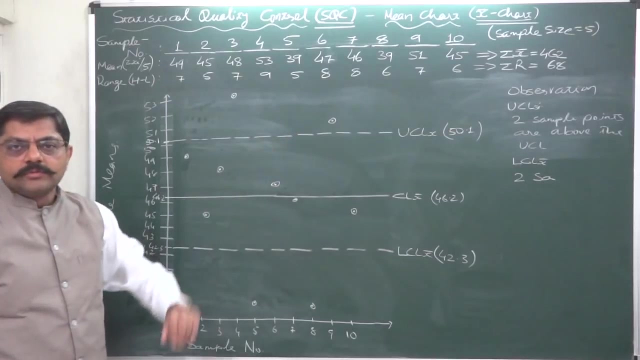 is to observe. is there any one or more sample points above UCL and below LCL? If there are, write the observation. If there is no sample point above the UCL and or below the LCL, then also write the observation. On the basis of this observation, we can draw the conclusion. 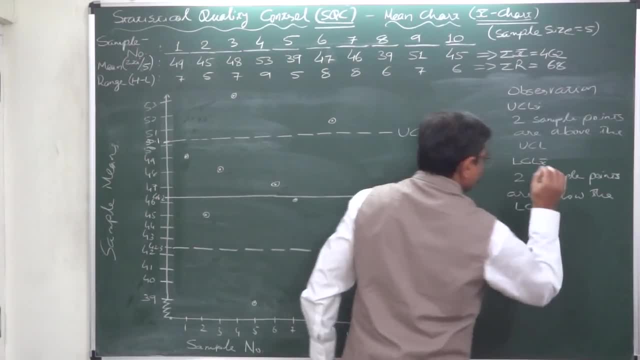 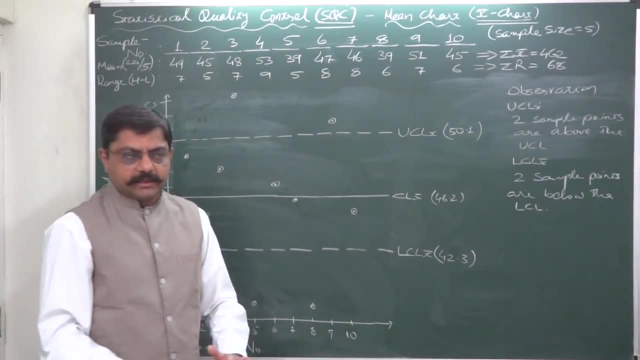 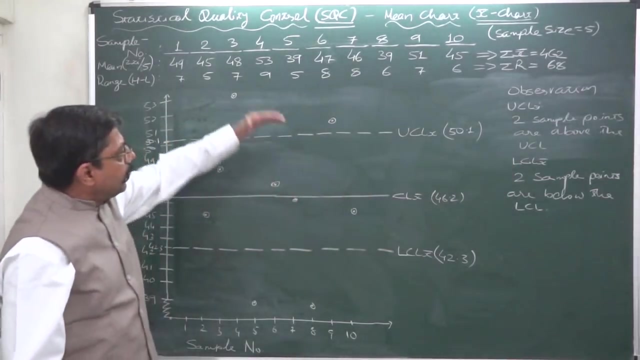 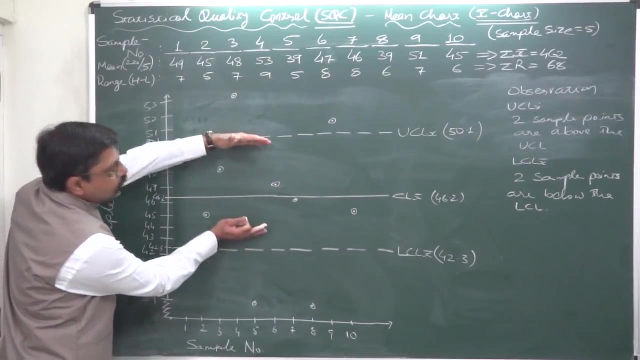 Now conclusion. What is the condition to arrive at or for arriving at the conclusion? If no sample point is above the UCL as well as below the LCL, that means, if all the sample points are within the two control limits, LCL and UCL, then we can conclude that the process 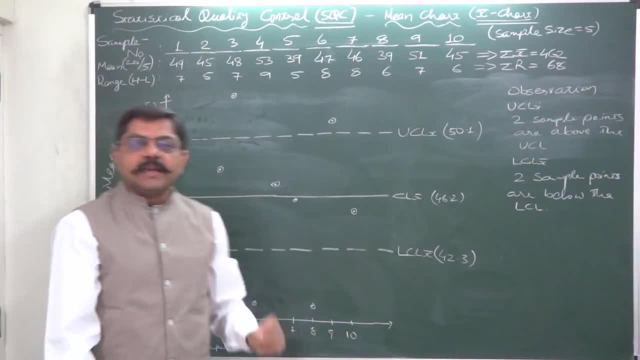 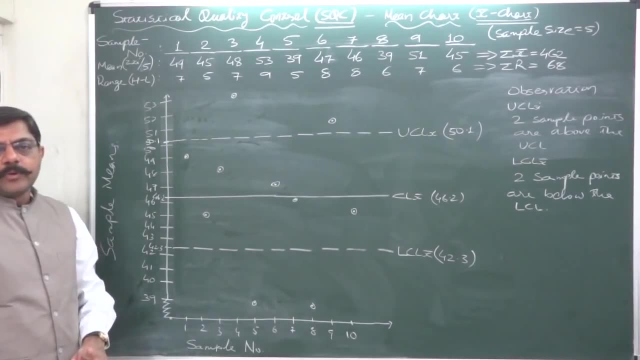 is under control. But if at least one sample point is either above the UCL or below the LCL, then we should conclude that the process is out of control. And here it is tragic. Out of ten, four sample points are out of the lower and upper control limits. Two are above UCL upper control limit. 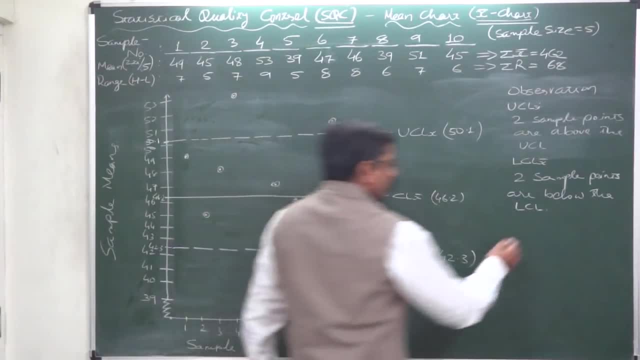 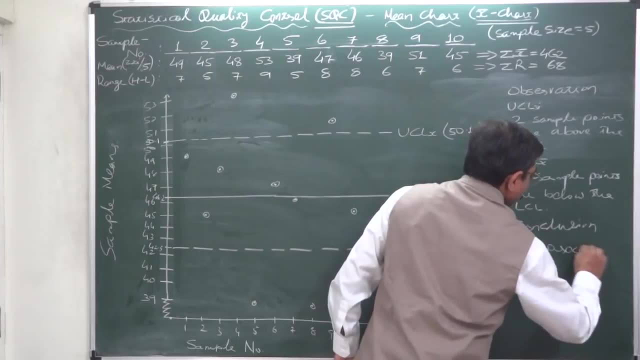 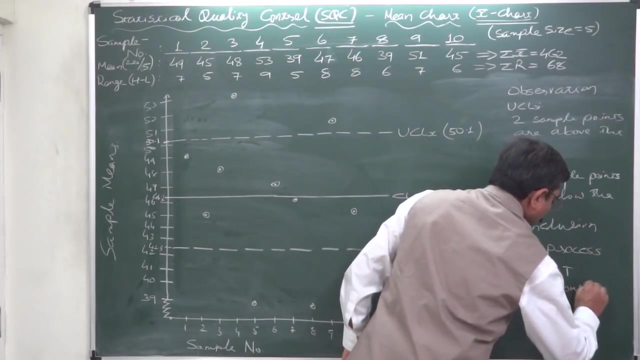 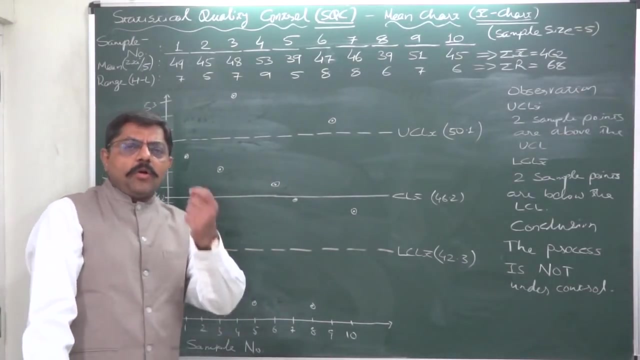 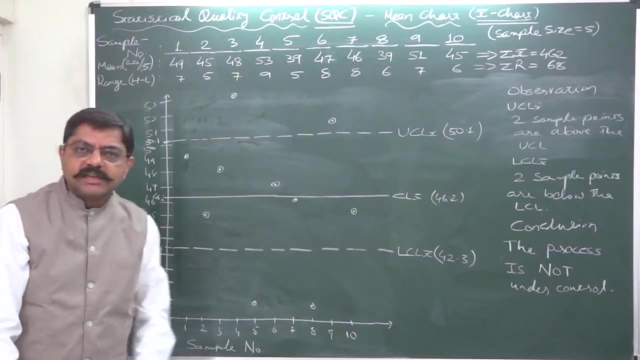 and two are below the lower control limit. That means the conclusion must be: 1. The process is not under control. The criteria is very much stringent, very much strict. Even only instead of these four, even only one sample point is either above UCL or below LCL, then straight away we should. 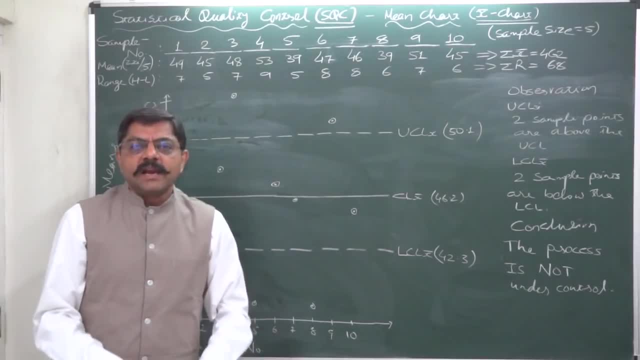 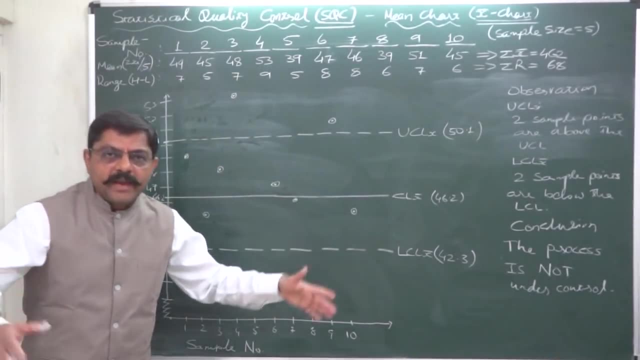 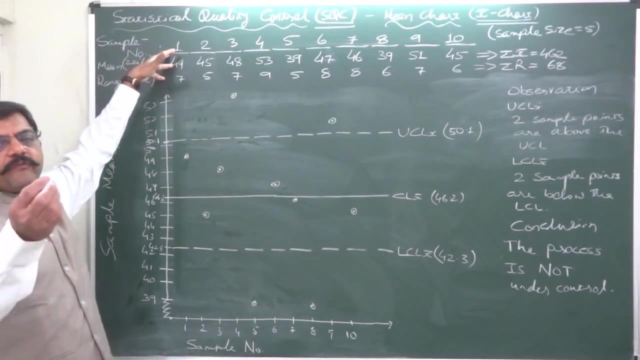 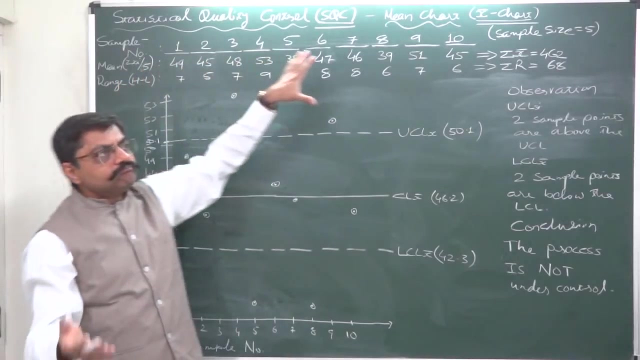 conclude that the process is not under control. Why? Why this kind of stringent criteria, or rather condition? Because this is based on sample From so many hundred or thousands of units. we draw the samples of, say, very few sample points. The sample size is only five. We don't know the population size, So we have to assume 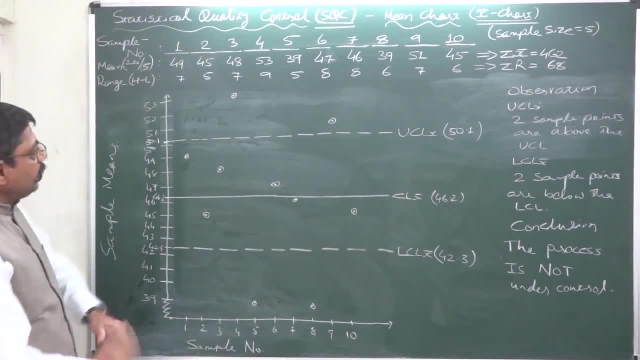 the population to be infinitely large. So from infinitely large units we have to assume the population to be infinitely large. So from infinitely large units we have to assume the population to be infinitely large From infinite number of units. we have drawn a very small sample, or say 10, very small samples. 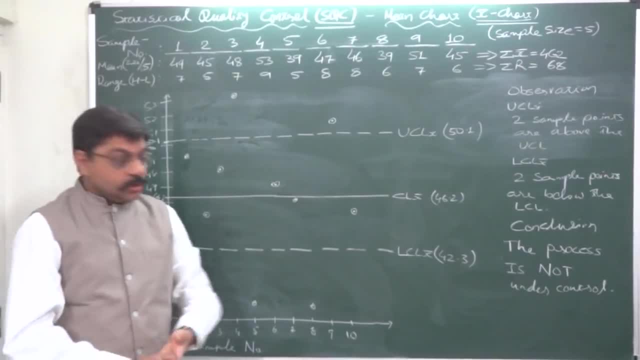 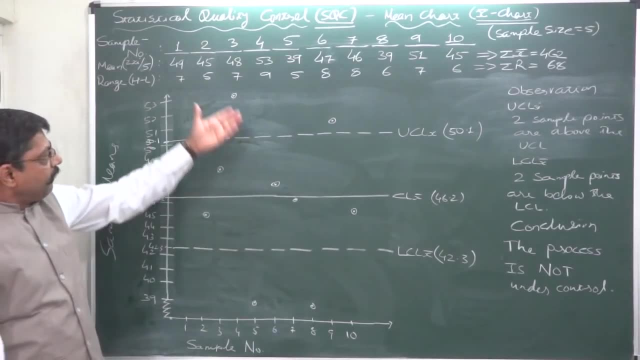 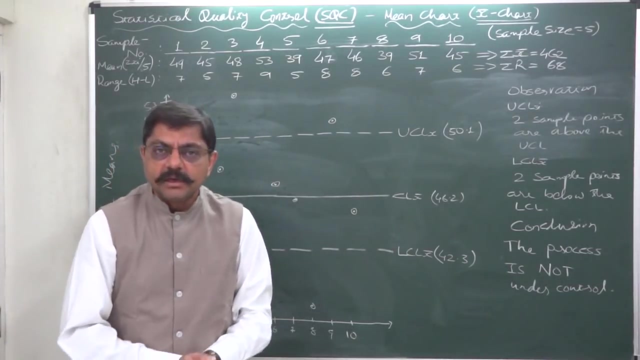 on the basis of which we need to arrive at the conclusion. So criteria must be very stringent and out of 10 very small samples, four are out of the control limits. Here it says this is one kind of exceptional case. Four out of 10 is a too much large number.